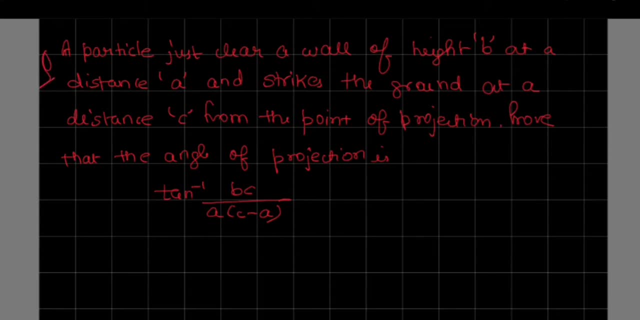 is stating: a particle just clear a wall of height B at a distance A and strikes the ground at a distance C from the point of projection. So you need to find out the angle of projection. It may be given it may not be. Then you just need to know about the method. So let's make 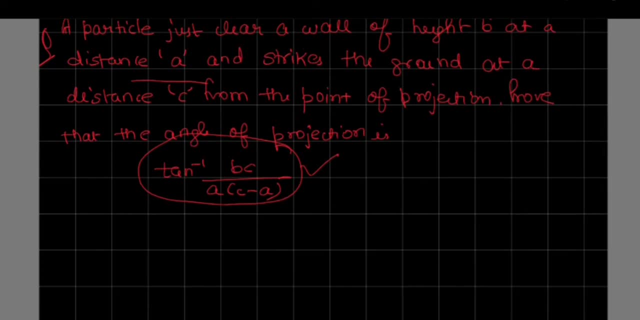 a figure. firstly. Firstly, a particle just clear a wall. Let's say, a particle starts from here and what happens here is a wall, Wall is of height B and when this particle strikes it it is at distance A from the wall. Now it just gets projected. It gets projected. so 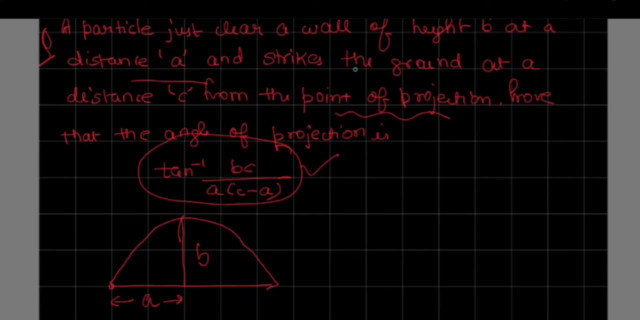 a projectile motion. that means a parabola, and the distance from the point of projection is a total distance. from the point of projection to the total distance, it is the value C, Right, A, B and C. Now we have to find out the angle of projection. So let's move on. 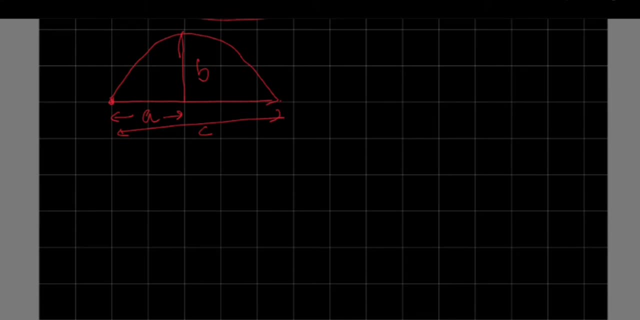 If you see. firstly, let me tell you about the velocities and its resolution. Velocity and its resolution. Let's say there is an article or there is a particle. It moves like this: Okay, it projectiles in this form. it has two types of velocities: one in x direction and another. 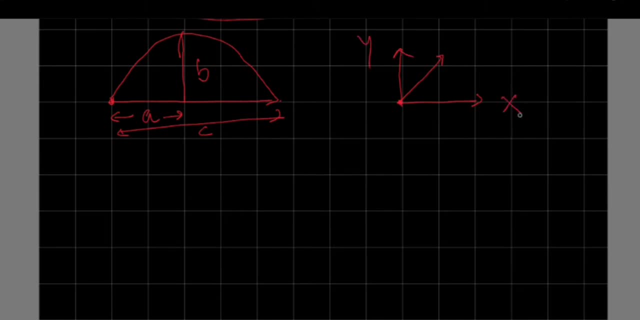 one is in y direction. so if the velocity of this is u and it is making this item, this particle is making the angle with x axis as theta, then the resolution of this vector will be u cos theta for horizontal component and u sin theta for vertical component. I am hoping. 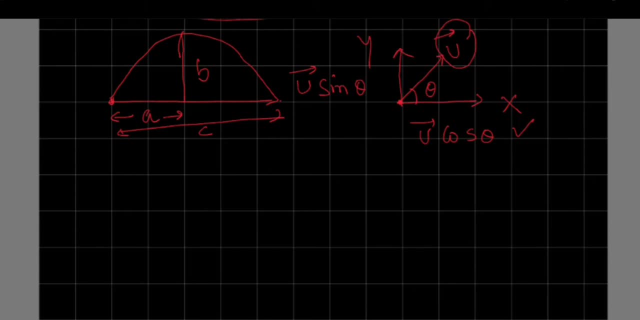 that you have heard about it and you have learnt about it before as well. so, similarly, let's say: if particle projects with this u, then the velocity, if it is like, if it is moving like this and it is making this path, So there are x and y axis, right, so let's start. if you see, this is your velocity in. 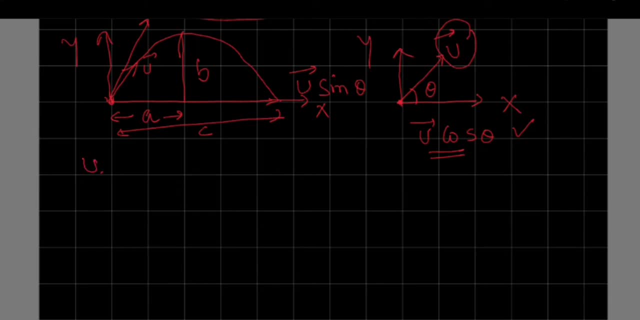 x direction. this is your velocity in y direction. so u x is u cos theta and u y is u sin theta. right now, if you have to find out the distance, let's say a or b, whatever it is. so a is your horizontal distance right. So what it would be. distance is always speed into time or displacement is velocity into. 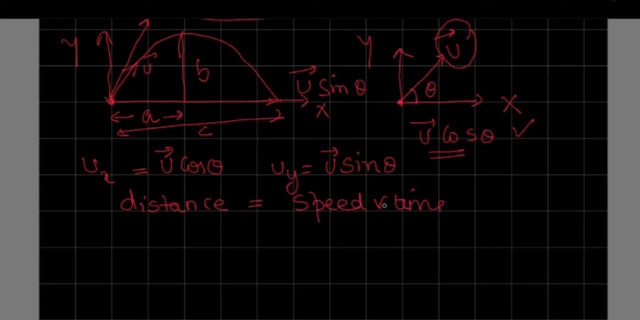 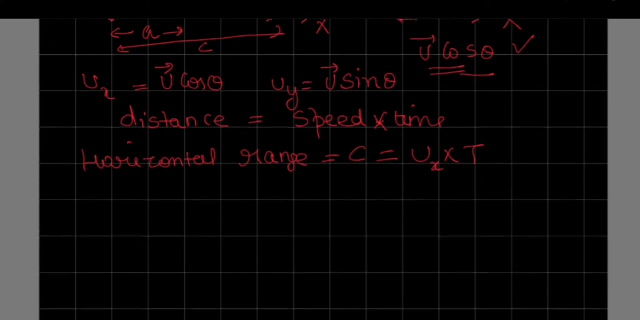 time right. so if you are talking about the horizontal distance, or you can say horizontal range, which is c here, horizontal range, it would be u, x, because it is horizontal. that means you will take horizontal component, u, x. or you can say let it be u x, t. okay, t is your total time, so here c will become u. 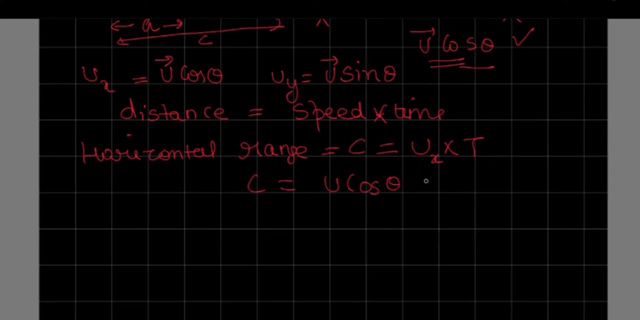 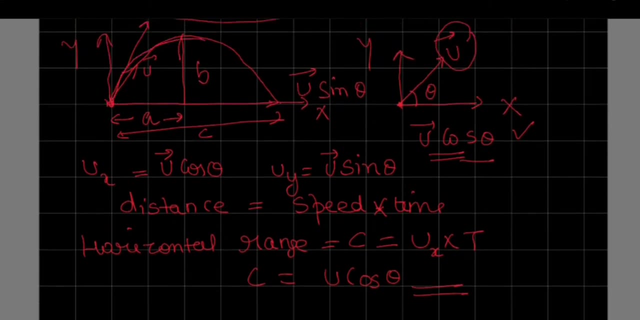 cos, theta and total time. let me tell you what it would be the total time, if you see, let's divide this total time of this particle, for this whole parabola, into two parts: one is for excision and another one for decision. So for this bit, only this bit. if you see, the maximum height which it can reach is b. 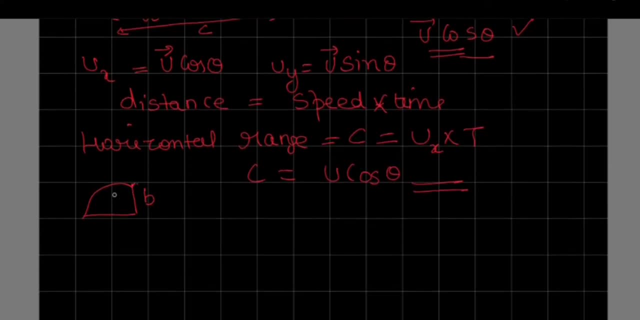 right. so maximum height is b, what you think. its initial velocity is u cos theta, right, but final velocity will be 0 because it will stop for a moment and then will come down for this path. only Now, if you find out the time time taken for maximum height, what it would be, So time taken for maximum height could. 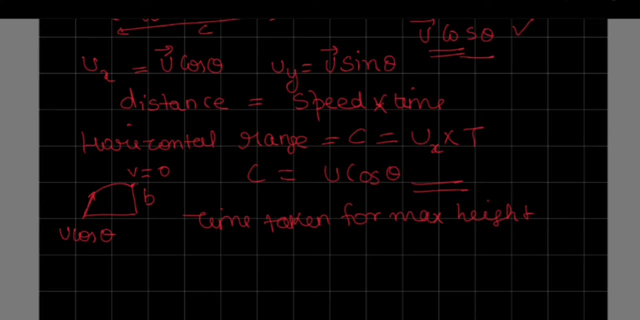 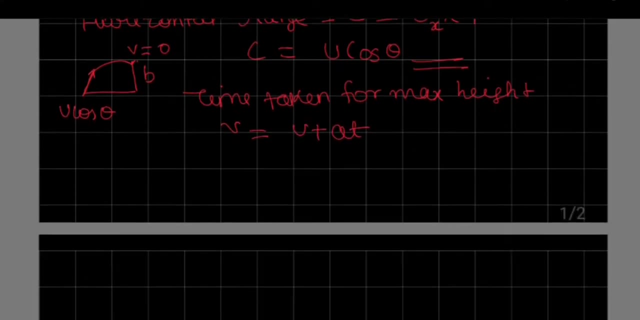 you please tell me for that v is 0, v is 0. So if you apply first equation of motion, which is v is equals to u plus 80, right Now a is acceleration. If you see here object is moving upwards, that means against gravity. So your acceleration due to gravity will. 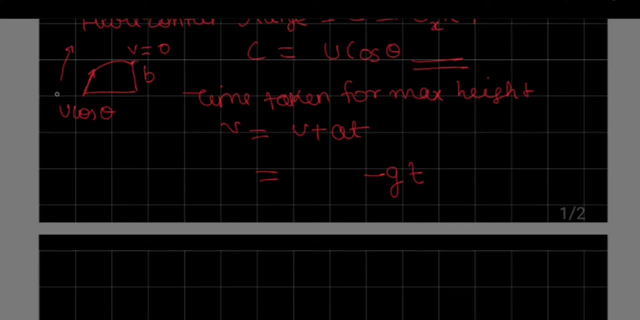 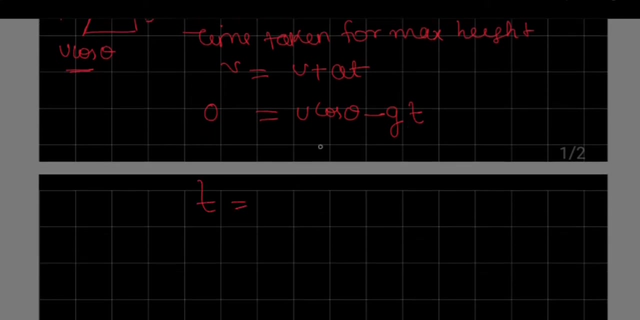 be minus g. Your time is t for this half circle. I mean half, you can say quadrant or half parabola. Then your v, because it is final velocity. so it would be 0.. Your initial velocity would be u cos theta. So time for accession only would be if you take gt left hand side. 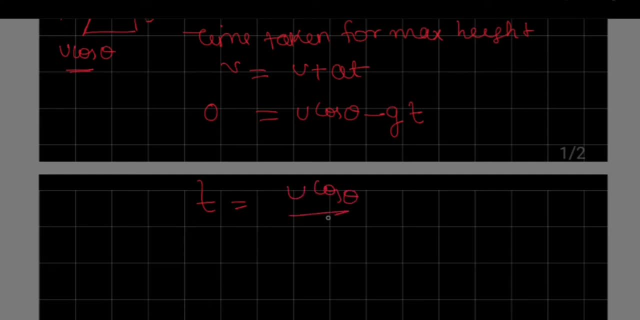 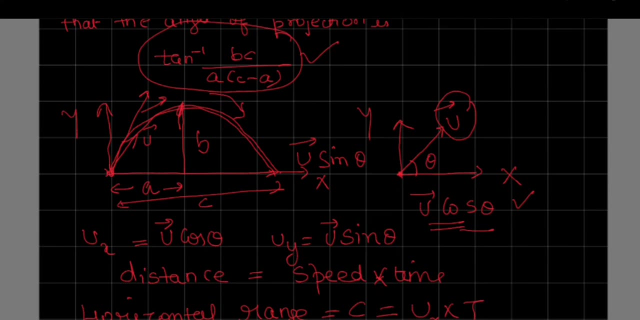 then it would be u cos theta by g. right Now, this is for only half path, So this is only from here. let's say origin. to this point let's say a. But you want for this time for horizontal range, you want whole time. So it will be same for this and this. 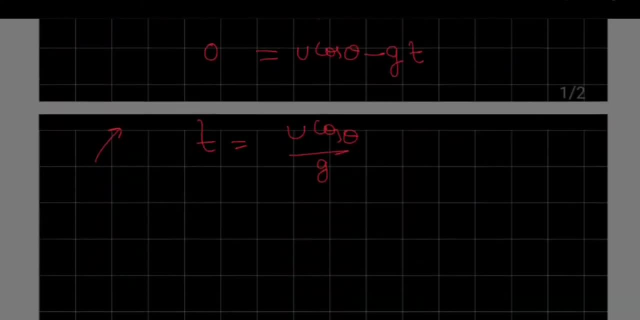 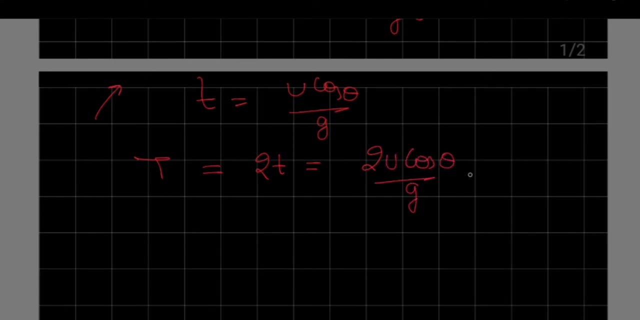 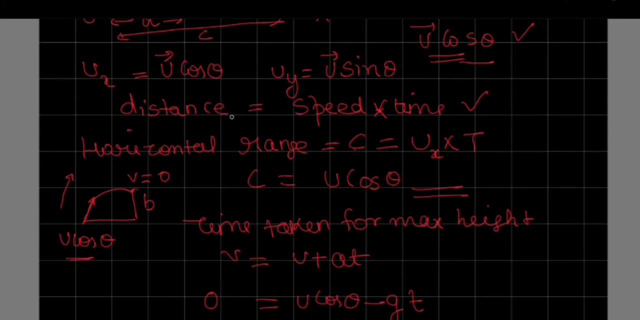 So total time will be twice of a session. that means total time period. Now this will be twice of t, that means 2u cos theta by g. Now substitute this value into here, into this equation, so your horizontal range, which was distance, feed into time u. 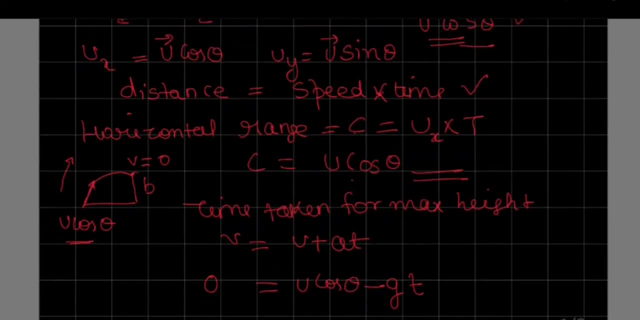 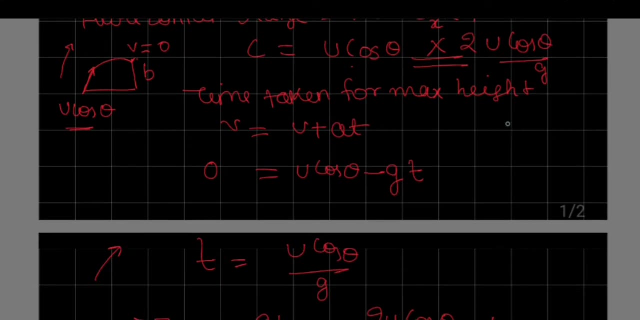 x is u cos theta. time would be 2u cos theta by g. Now you see, if you solve it, it would be 2u cos theta by g. It would be- let me erase it- So what it would be. 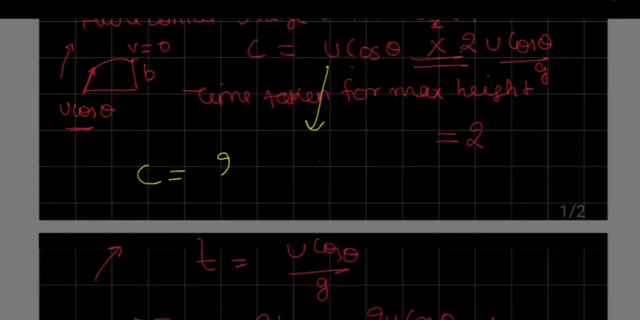 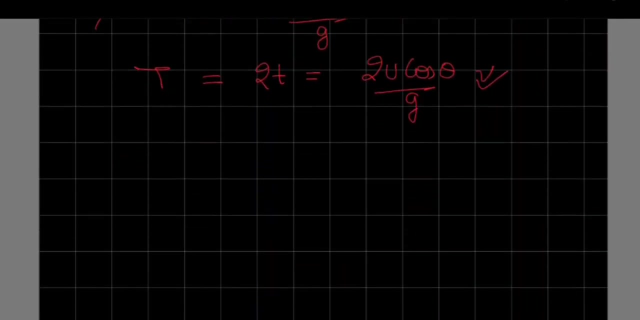 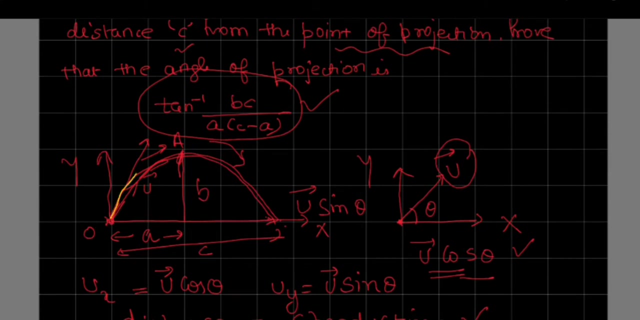 Here C would be 2: u square cos theta. I mean cos square theta by g, Right? So u would be like this, And let me tell you this bit: This was one thing we got in error. If you see, here it is moving up right. 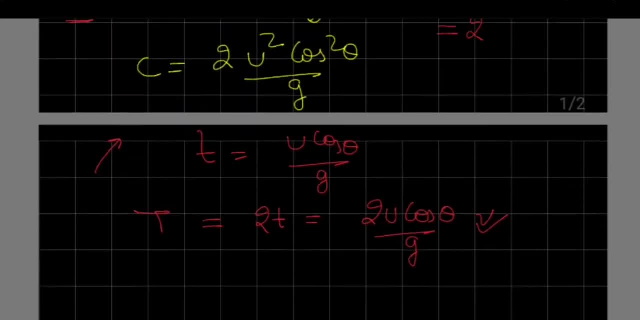 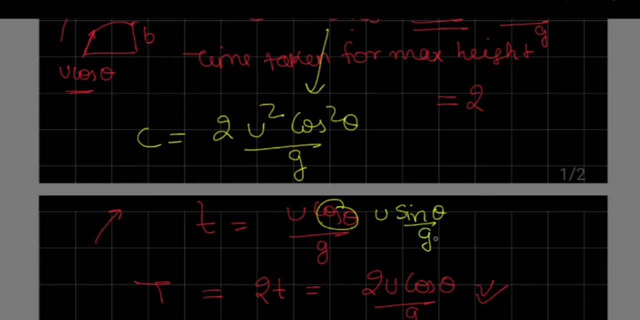 So time for a session here. it would be see, here It should be. the velocity should be u sine theta, right Because it is for vertical, vertical axis, Right Because object is moving here. So you will see, you will take the, you will take what. 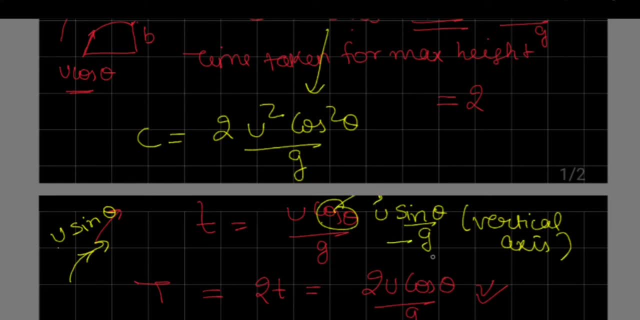 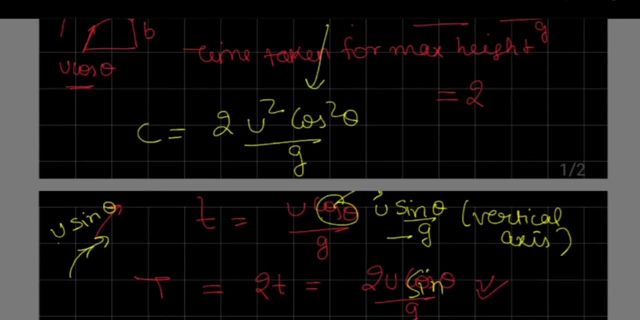 Vertical axis u sine theta. So it would be u sine theta by g. That means, once you put this value here, that means 2 u sine theta, And it will take 2 u sine theta by g. So now, if you see, 2 u square. 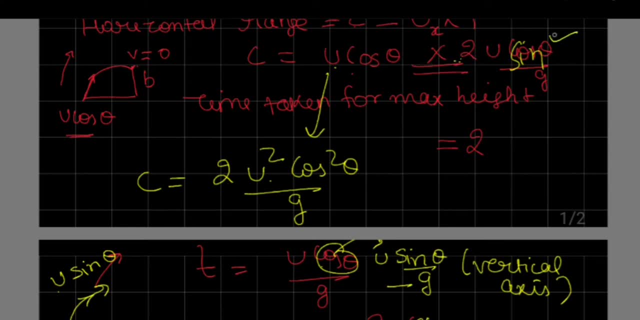 If you know the formula 2 sine theta cos theta, What it is for trigonometry, Let me okay. So if you know the formula 2 sine theta cos theta, It is sine 2 theta, right. So u square by g, it is sine 2 theta. 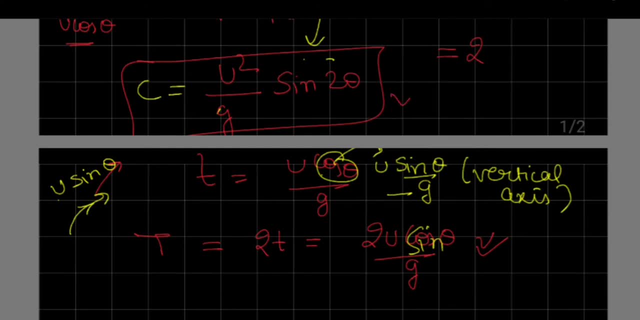 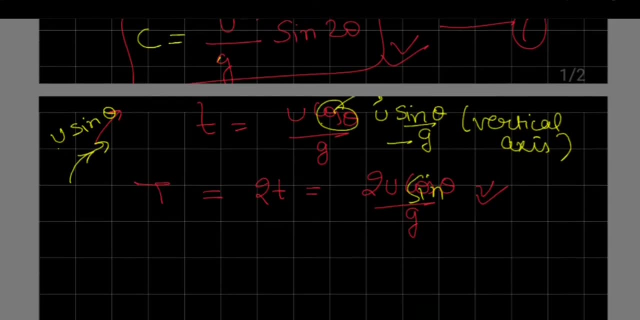 Alright, So it has become: this is your horizontal range. Alright, Now moving on, you have to remember this. Let's say: this is first equation. Now, if you, if you know the second equation of, of motion, 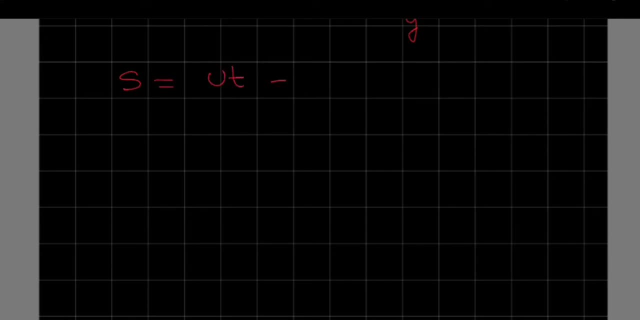 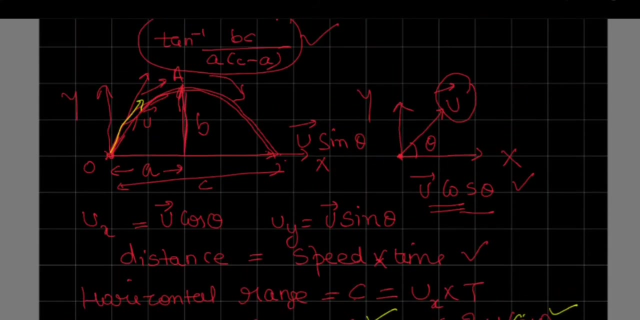 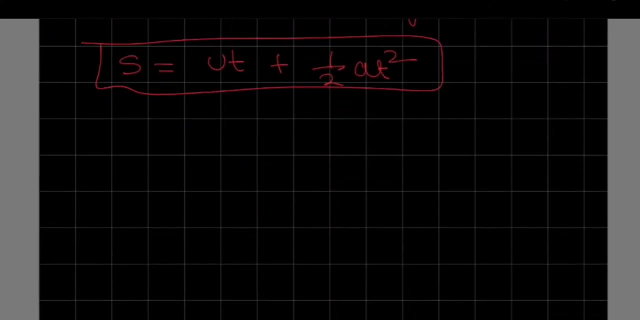 What is it? S is equals to u t plus half a t square right. So if you want to know about this vertical distance, this b, what it would be Vertical distance: this is second equation of motion. Substitute all these values. 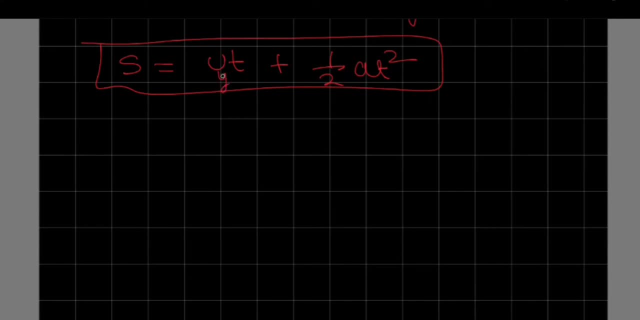 Because we are Going vertical. That means you will take the just assume everything and presume it in the form of direction. So, because you are taking vertical axis, so it will be u, y And acceleration will be against gravity. 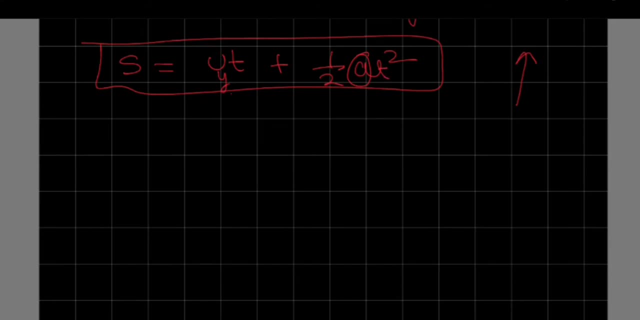 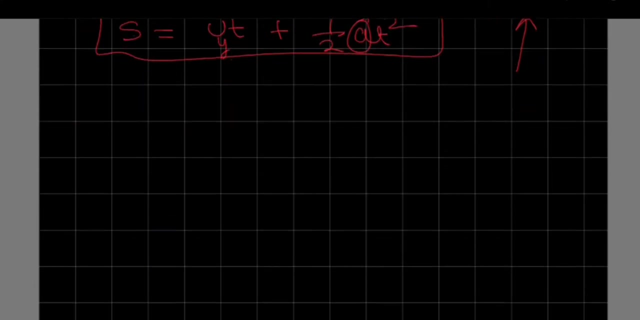 Okay And time will be half. Okay, You can consider it. and this is: this is vertical, which is b. So b would be u sine theta, T minus, because acceleration is against gravity. so a would be minus g, so half g t square. 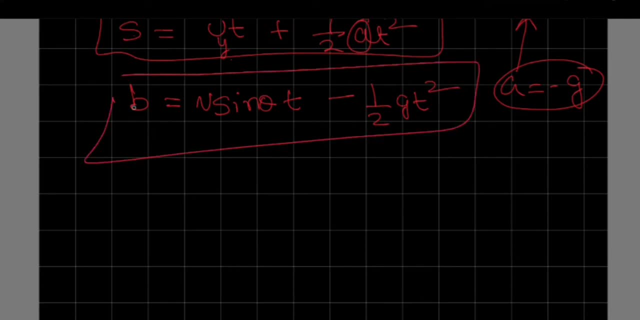 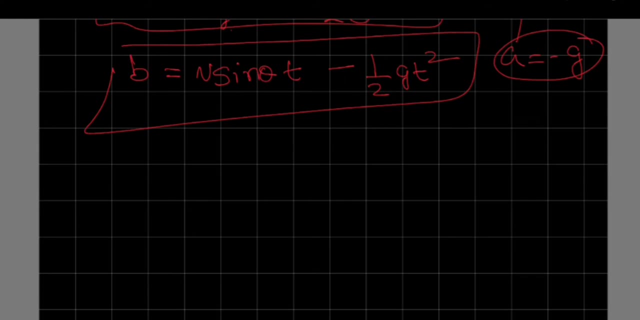 Alright, So b would be this value. Now you have this, I would like to ask you what? what would be the value of? if I ask you the value of u? You know acceleration, or we can say distance is speed into time, simply. 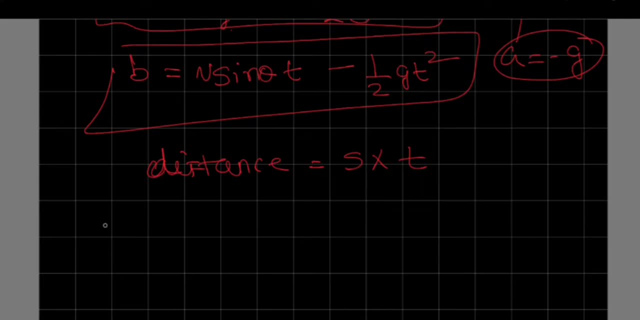 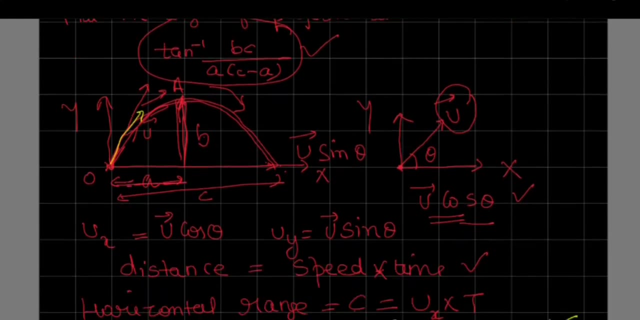 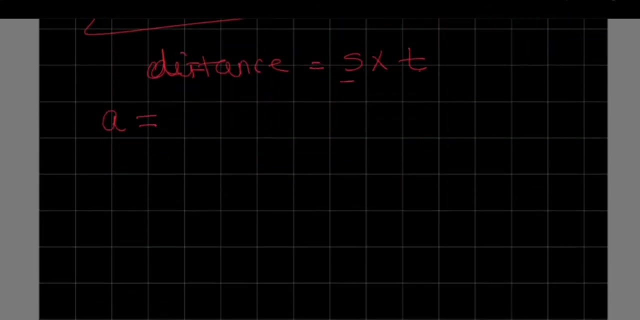 Right. So if we talk about distance in x-axis, distance in x-axis, which is a here in the figure a, and distance in y-axis is b, so a would be speed into time, a is horizontal distance. 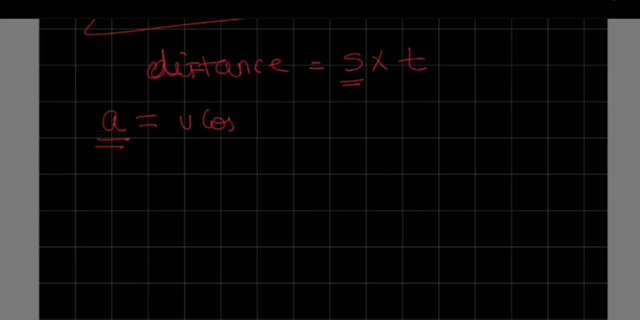 so horizontal velocity, which is u cos theta, into t Right. Similarly this was for horizontal. If we take for vertical, then what it would be Distance for vertical is b speed, u sine theta and t Right. So this is similar. however it would, it would be having this bit as well. 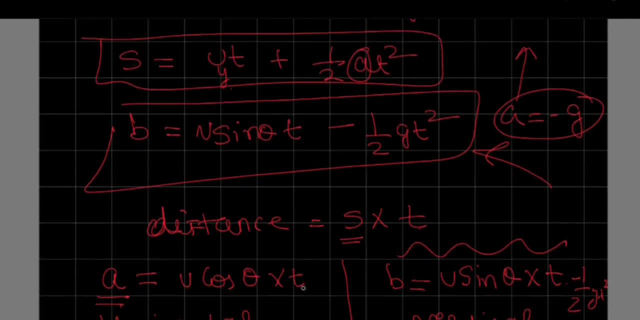 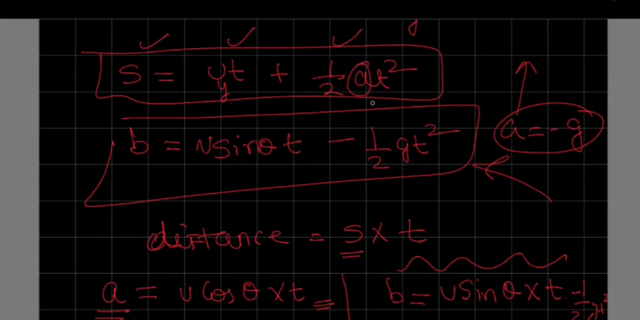 Why? if I ask you why we didn't take anything here? Because the formula is this: s is equal to u t plus half e t square. but for horizontal it's a straight line. because it's a straight line right. 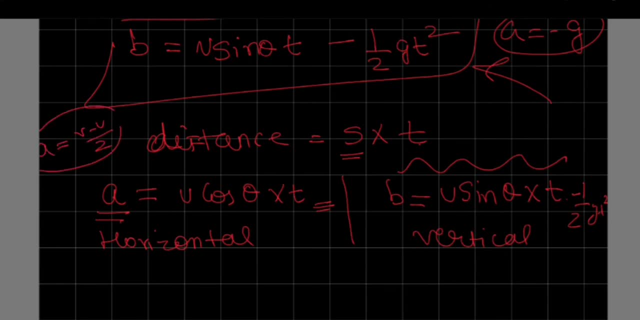 So if we plug in with this, that's going to be, I'm going to find out that this is the energy. So this is the energy and it's going to be constant, not the velocity. Now let's take a look at the x-axis. 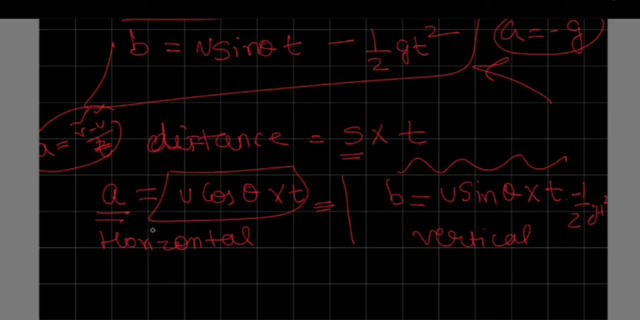 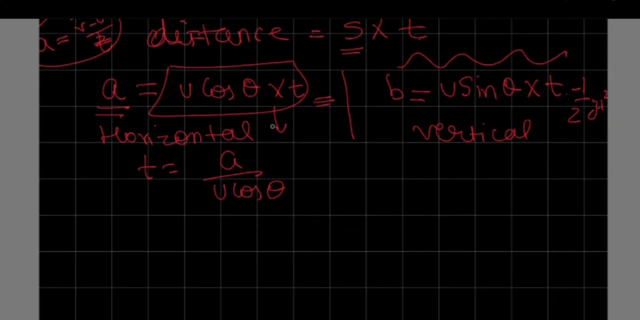 So is the velocity constant. So that is the value of x. Okay, So if we take the, let's take the x, What is it? Okay? and from if you substitute this value into this equation, okay, so what you do, what you will get. 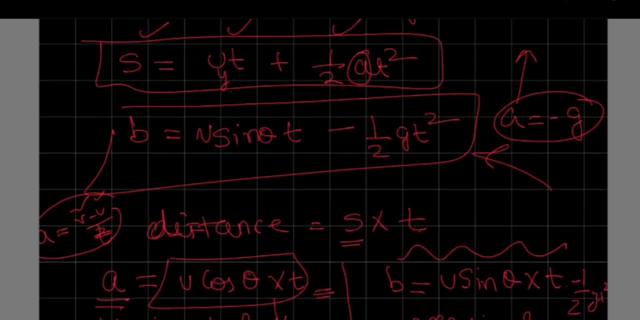 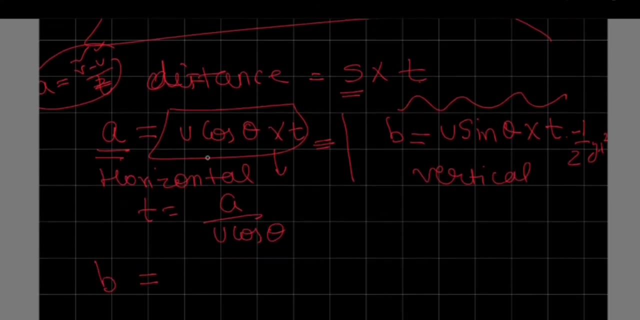 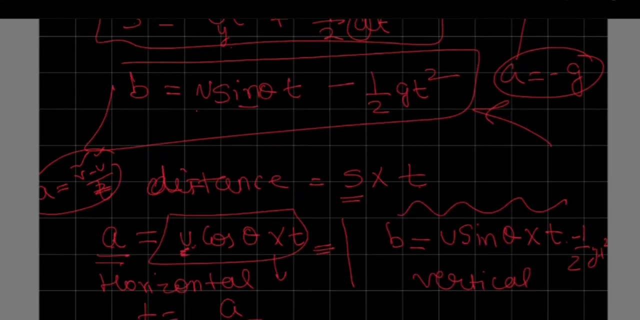 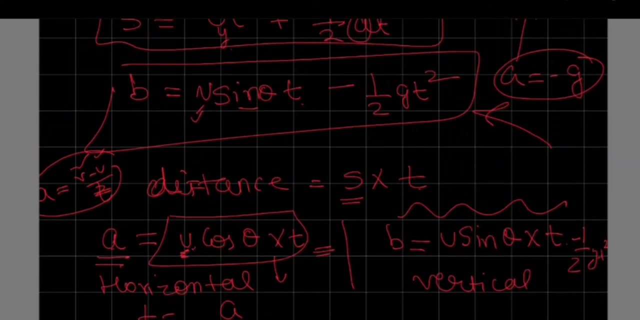 b is equals to c. this is u, u sine theta t, right. so the value of u, if you take from here the value of u is a by t cos theta, right, so a by t cos theta. okay, then here you have substituted value of u now sine theta t, right. then you have minus half gt square, so minus half g the value. 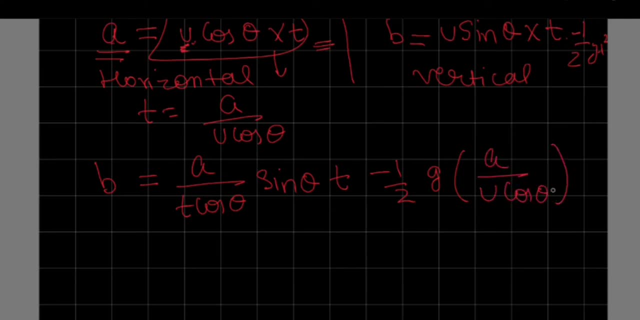 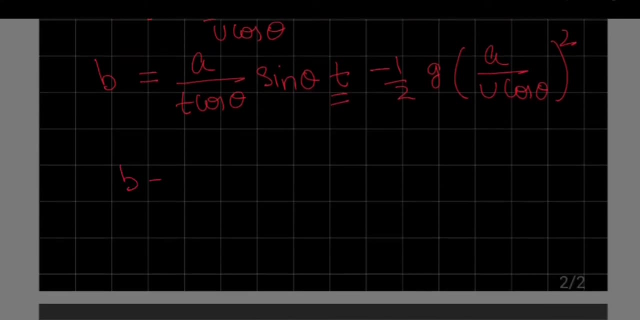 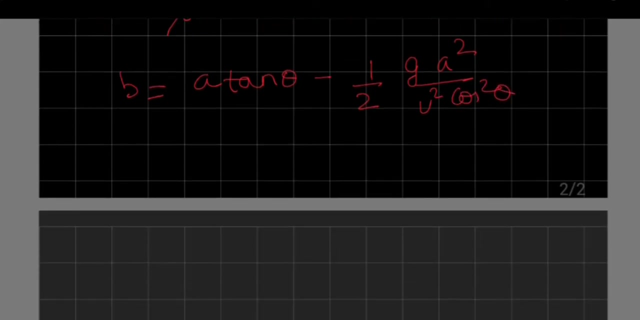 of t. is this so square right? here also you can substitute the value of t. but before that let's do this. t is cancelled with t. a sine by cos is 10 theta minus half g. a square by u, square cos. square theta right. so this is one of the value. if you want to simplify it more, then you can take it like half. 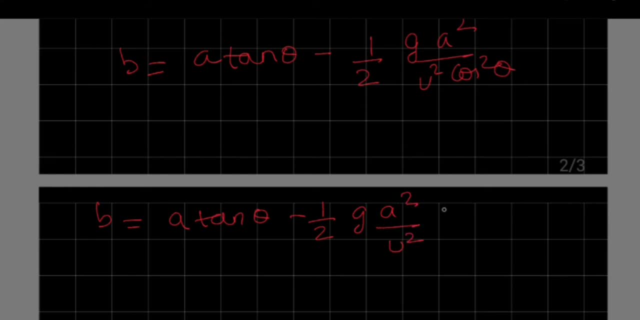 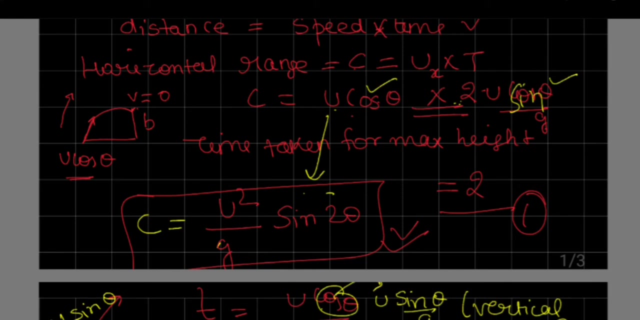 g. a square by u square one by cos is sec, so sec square theta. now you have value of b like this. but if you remember what's the value of c which we got for horizontal range, this value right c, is equals to u square by g, uh, sine two theta. so from here we can see that the value of anything like, if you want the value, 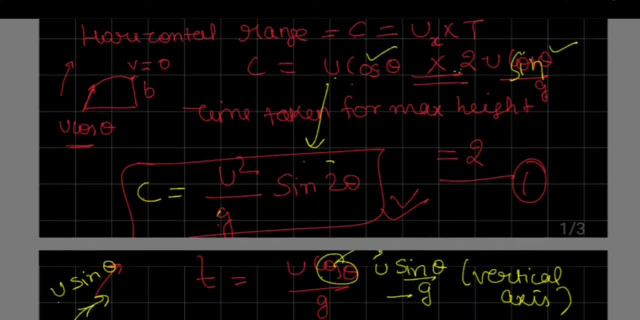 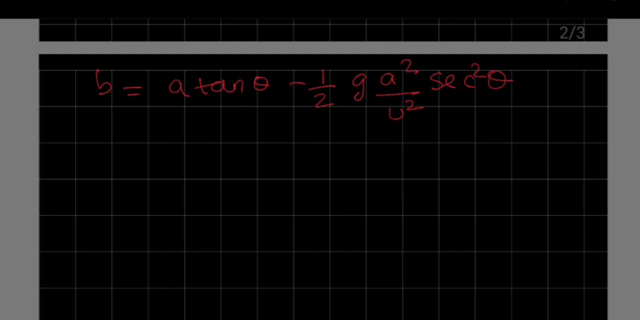 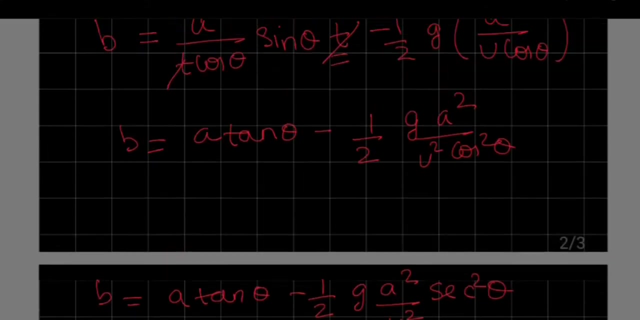 of u square, then we can have c g by sine two theta, right, we can substitute this value here. so we have b- a disappointment, minus half g a square by u square. so substitute that value. this is a ten theta minus half. so g a squared sec square theta is okay, but the value of u square is value of u square. sorry, 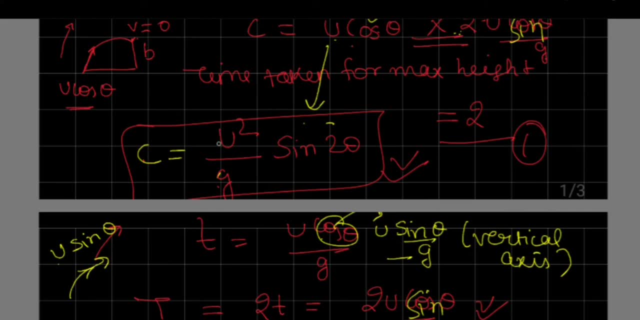 that i have to go up and down all the time, uh, but i'm hoping you are listening and u squared is。. second vs z: prime of t is equal to north cross between both ends of thing. therefore that is another. говорю kilkaah empezakar Schrittquietane poit 입ерж dunfie verses their toант. 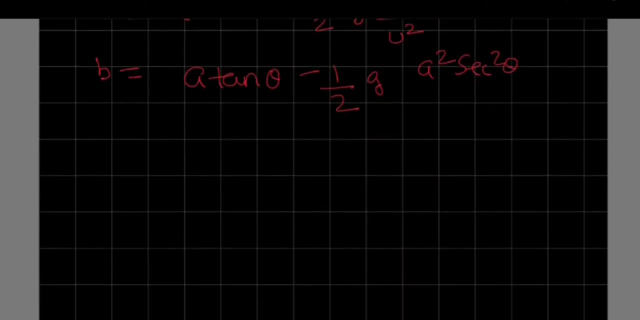 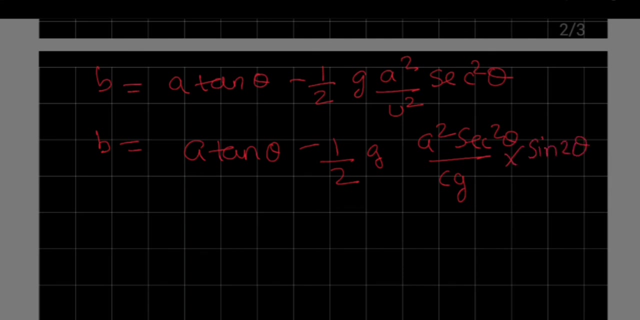 is CG by sine to theta, right CG by sine to theta. So u square is CG by sine to theta. Sine to theta will come up right Now. solve this equation and simplify it. You have g's. cancel the g and then, if you know, this is minus half a square by c. Sec is what 1 by? 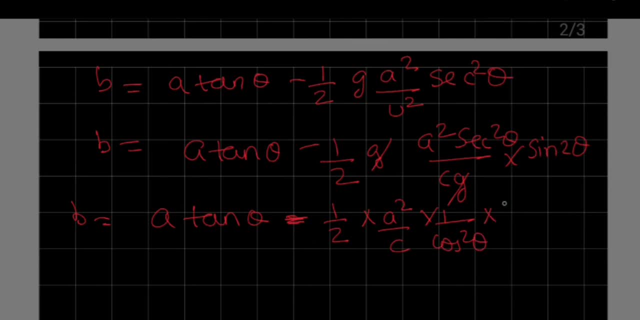 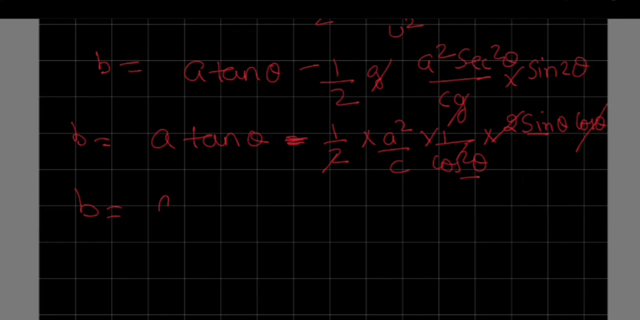 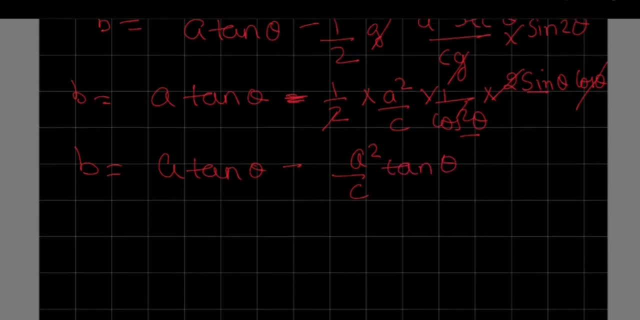 cos square and sine is what Sine to theta is 2, sine theta cos theta, 1 cos is cancelled with 1 and then sine upon cos is again 10.. 2 is cancelled with 2 and sine upon cos is 10.. So a, 10 theta minus a square by c, 10 theta. right, You can take LCM C Here a. 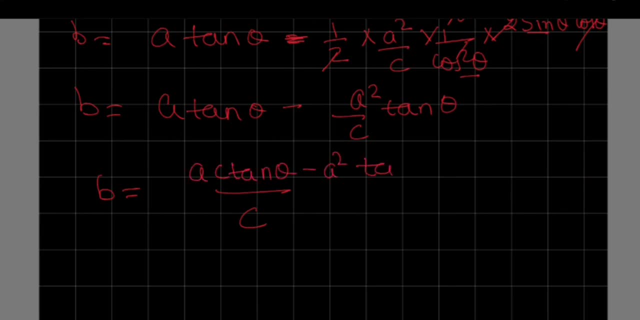 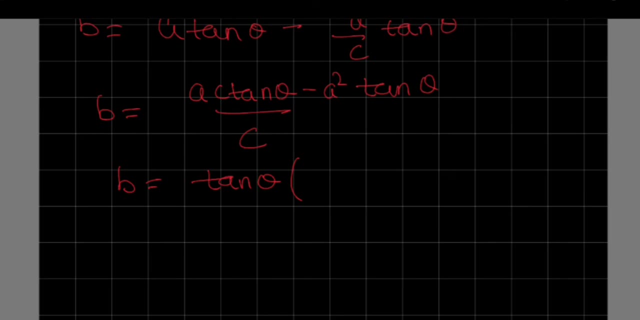 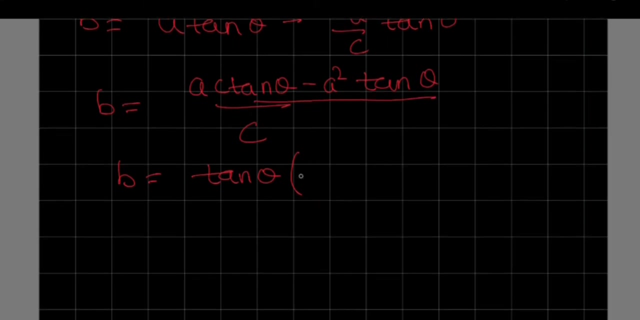 c: 10 theta. So a 10 theta minus a square 10 theta. you can take 10 theta common and what you have got. So you have got here, this is all with it. So 10 theta is common. You can take a. 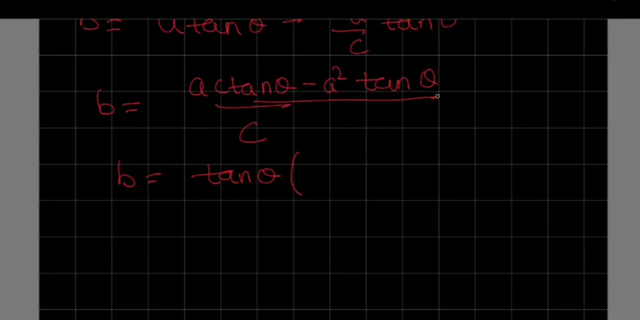 as also common. but this is a c 10 theta. If you take 10 theta common, what you have got a, c minus a square by c, right? So take this here: b, c, Take this in denominator: 10 theta. You can take a, also common, c minus. 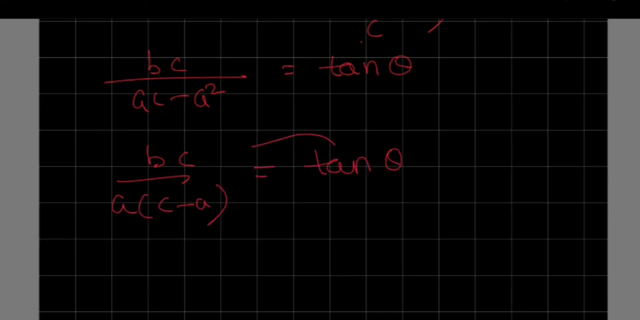 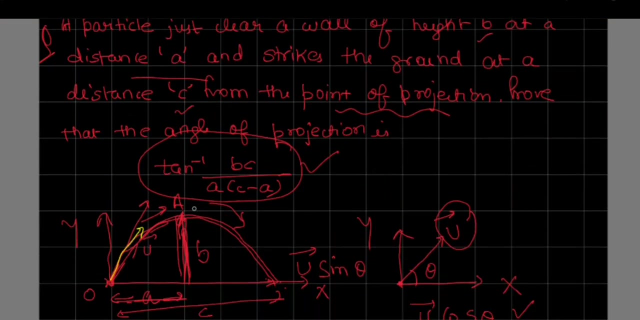 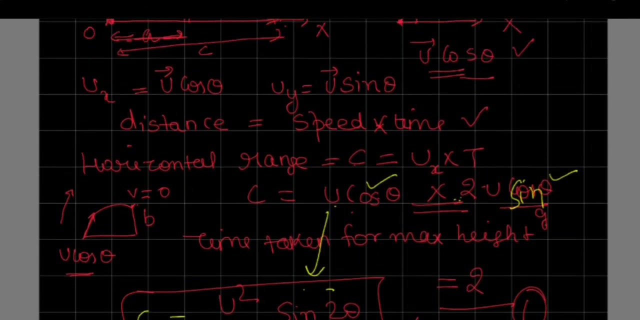 a 10 theta, and if you take 10 there it will go in inverse form right: 10 inverse b c by a c minus a. Let's see, is this what we were supposed to prove? So see: 10 inverse b c by a c minus a. So remember, you just need to know some trigonometric formulas. 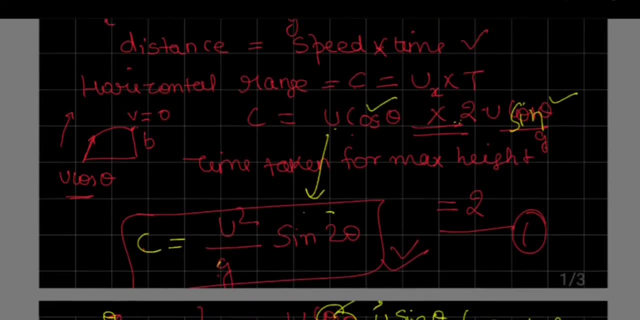 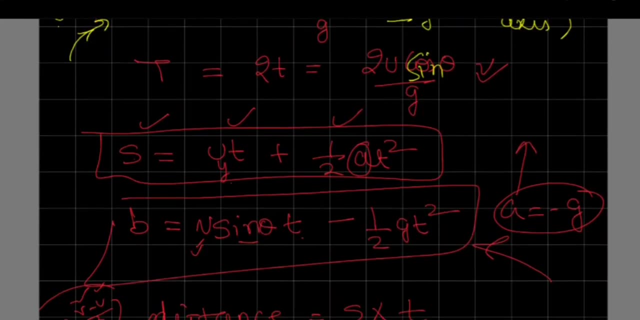 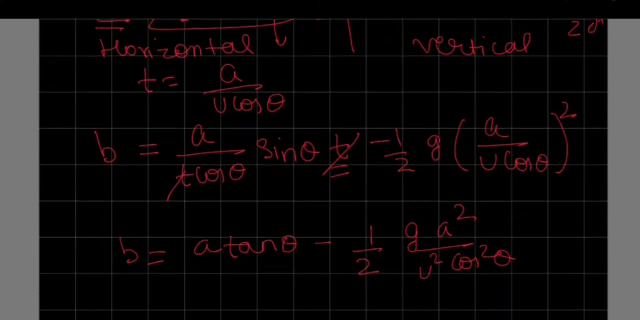 and what Some? some motion equations of motion. So second equation, we have used u t minus u t plus half a t square for distance. and first equation we have used and the general formula which is distance speed into time, All these formula you should know about sine. 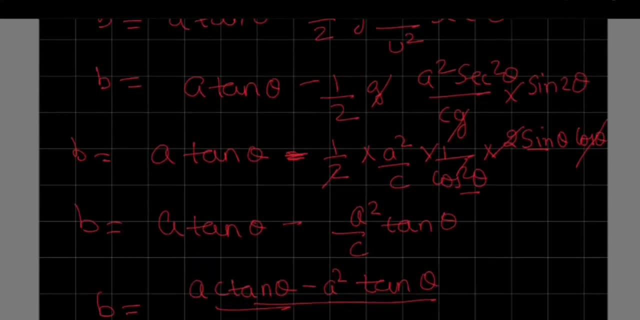 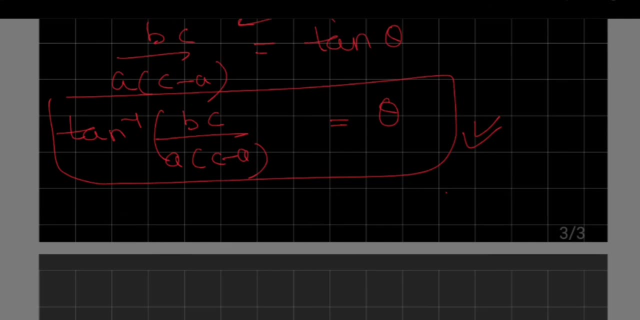 upon cos is 10 and then inverse of cos is sec. Some of the few formulas, and then you have got this. I'm hoping that you've understood it and if so, then don't forget to like, share and subscribe my channel. Take care to my. 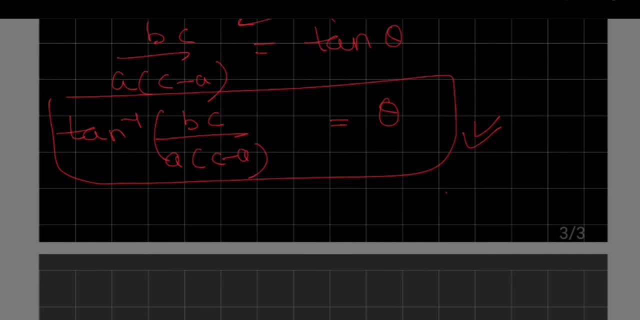 next class and I'm hoping to have so many comments from you all, guys, and I know this time is hard, but stay safe. stay safe and keep yourself calm in these hard times. Prepare yourself for your studies and let me know how many topics you're finding difficult.